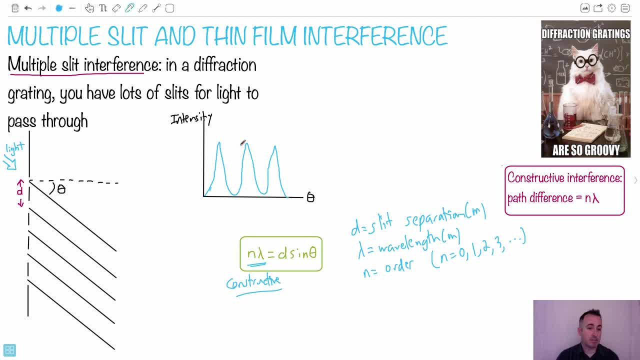 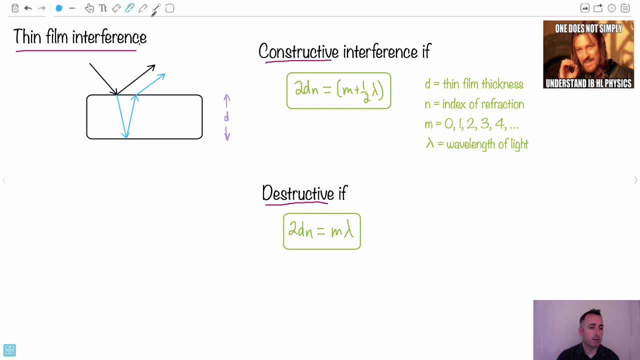 like this. Now, this right here will be your peaks. I think that's about all you really need. So let's just take a look and see if we can do the next equation, which is within film interference, And then we'll see an example. 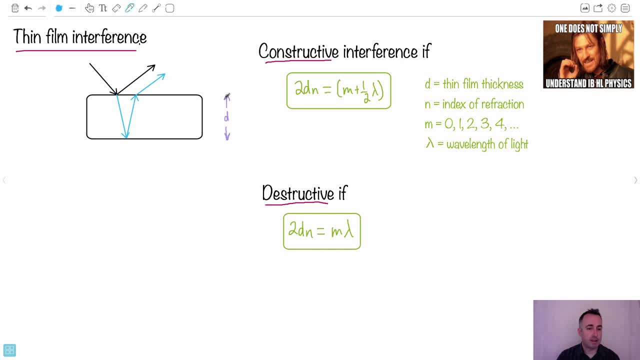 So here, if we have a thin film, what we have is: we have a thin film, We'll say the thickness of it, we'll call it D, So that will be measured, of course, in meters. I love this. One does not simply. 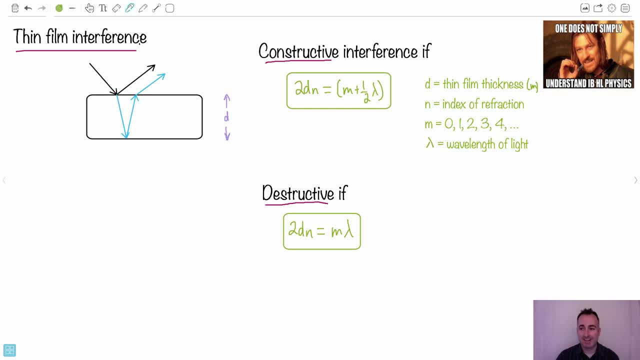 understand IVSHL physics. That's from Lord of the Rings, right? This guy always dies in movies, doesn't he? Or shows Like in Game of Thrones in the very first season, right? But anyways, we have an N. This gets a little bit confusing, because in the past we've often been using these. 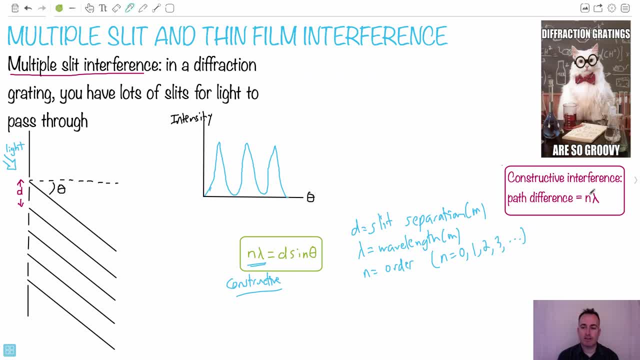 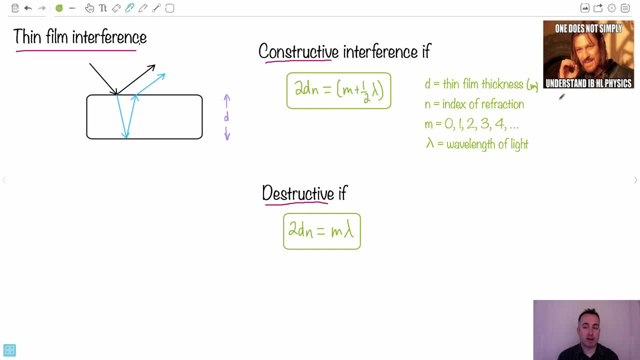 order, So we can say like 0,, 1,, 2, 3.. N has always been this order. Here. however, they've got M being the order where N here is the index of refraction, So just watch out for that. That's the. 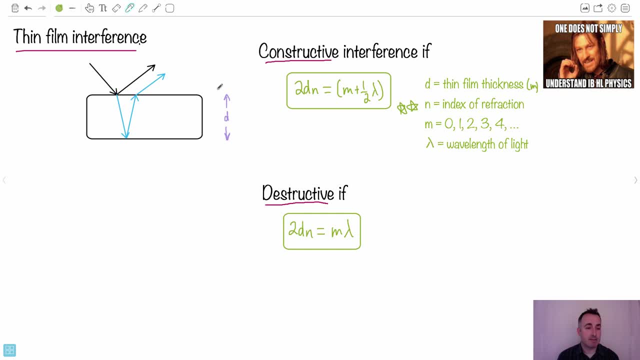 difference between N and M. This N changes. It becomes the index of refraction of this light, not this light, this material, whatever it's passing through this thin film here. So M can be 0,, 1,, 2,, 3,, 4, whatever numbers you want, And lambda is the wavelength of light. 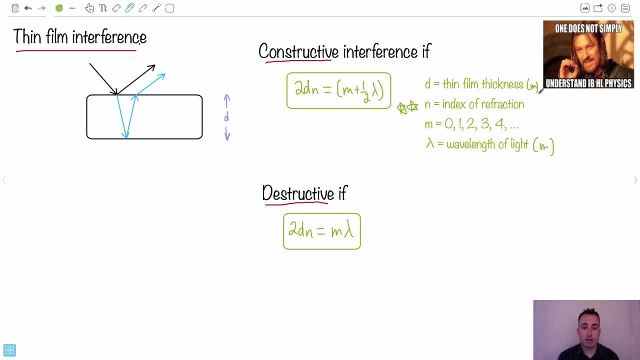 which is measured in meters And index of refraction has no units. So we end up with this equation right here that we have constructive interference. We say if 2DN equals M plus a half lambda. Now we also have destructive interference if 2DN equals. 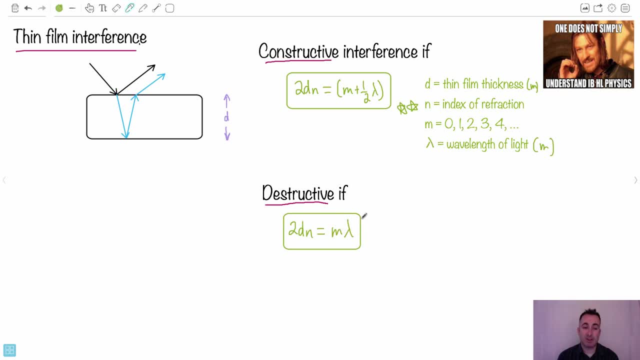 M lambda, Basically, you just have to look at what it is that they're giving you and you can figure this out. What's really going on is we have light, like one beam of light here, one ray of light. It's coming in and it's reflecting directly off that surface. 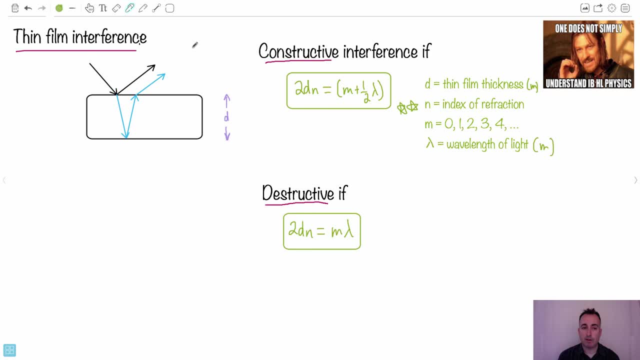 this thin film, So it reflects directly off There you go. It's received somewhere over here. We have some of that light. however, will go through that into this material here, into this thin film, And of course it will refract. So maybe, for example, 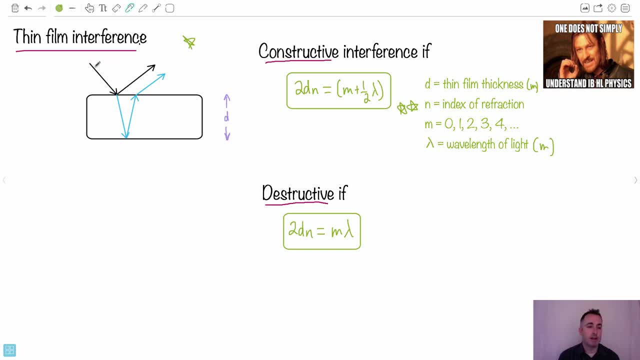 this thin film had a higher index of refraction than air did, Then it'll do something like this: It will slow down. So that means remember we learned about this in topic four. The angle here in is: this angle here is smaller than that one. I guess it slows down. 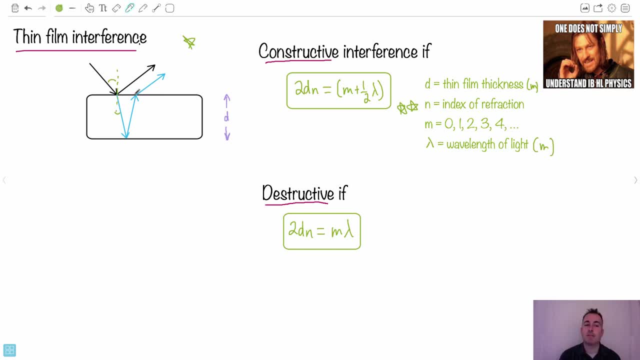 And now we can say: great, it does that, Then it bounces off, and then it does the same thing, except now it refracts on the other way around. So here, if you look, the angle is very small. Now it becomes. 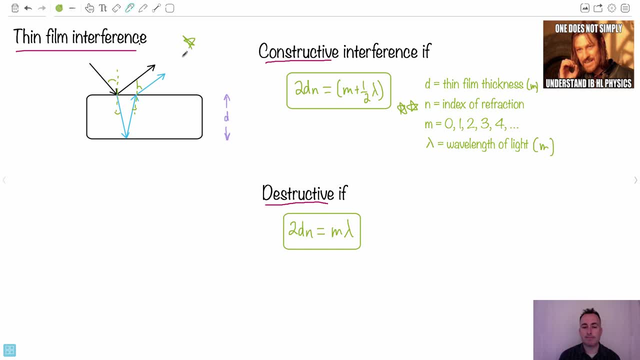 bigger And these endings end up hitting parallel like this. So you can basically talk about where you're going to have peaks, which is destructive, constructive interference, and where you have dark spots, which is destructive interference. Actually, that's about all. you need The theory. 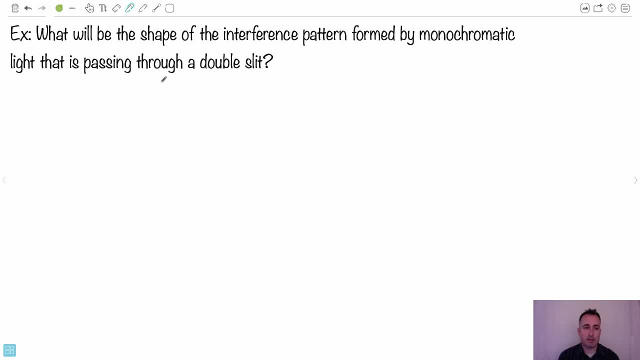 you really need for it. Let's see. Now we're going to deal with a couple of questions here. First of all, what will be the shape of the interference pattern that's formed by monochromatic? remember that just means wavelength equals just like just one number light. 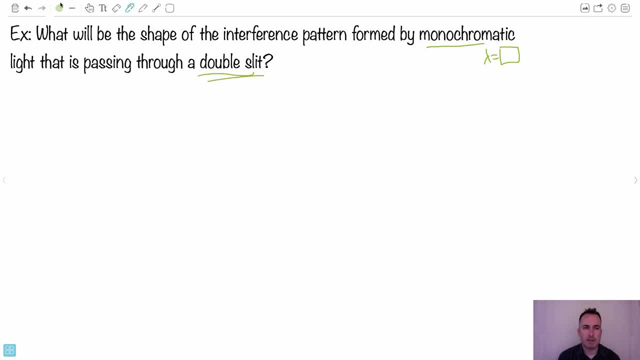 that's passing through a double slit. what happens is, if you have a double slit, what we can do is we can maybe try to draw the try to draw the interference pattern here. what will happen is this: you're going to have a single slit thing right here that's going to modulate this double slit thing. so you have basically: 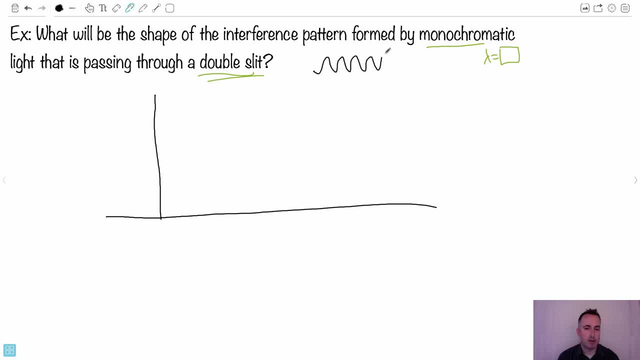 multiple slit interference. remember that. I mean that wants to do this sort of shape, but it's going to be modulated by this single slit thing. so remember the the shape of a single slit diffraction did something like this, like that, so what you can end up having. it's gonna look kind of weird, but watch this. 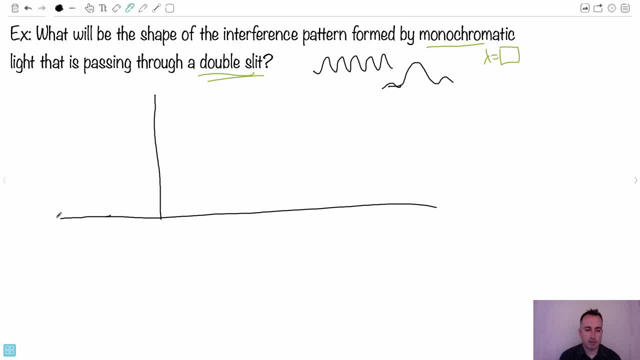 carefully. here you're gonna end up having. this is in the center. I guess let's do it like this, so here can be theta. this could be the intensity we could say it's gonna look like what's very, because it's gonna be kind of cool here, so you're gonna see it go kind of up like this right here, and then this: 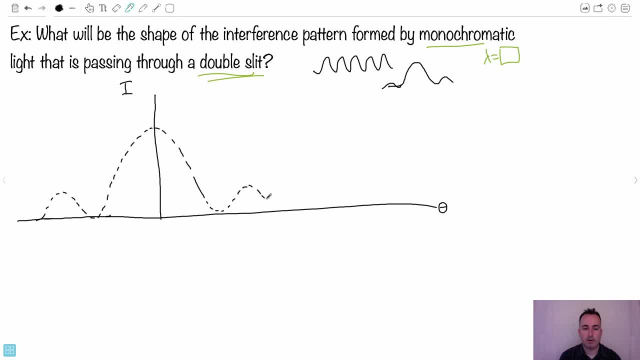 thing is gonna go down like this: I'm drawing. it's gonna go down like this: I'm drawing. it's gonna go down like this: I'm drawing dotted line for a reason, because what's gonna happen is: you want to have this kind of shape, but you also want to have this kind of shape. so what you're gonna 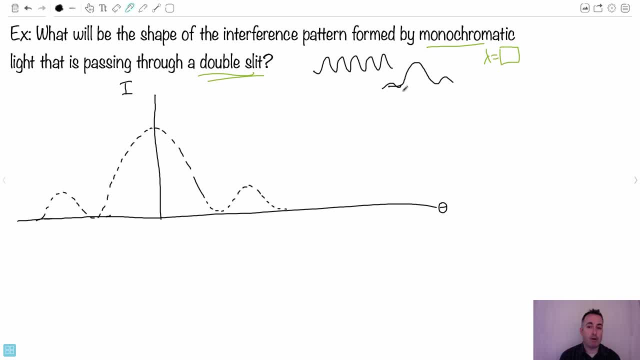 do? you can have all these little squiggles like this, but they're gonna be sort of bound by this thing. that's what I mean by modulated by. so now it's time to have a little bit of fun here and try to draw- maybe different color, I'm gonna. 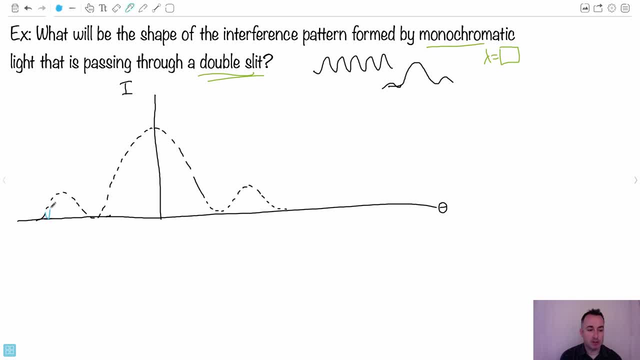 try to draw some little squiggles that have to fit within this. I'm just gonna just start to draw squiggles here. it doesn't have to be exactly something like you know. this right here I'm gonna go up and down and up and down, like: 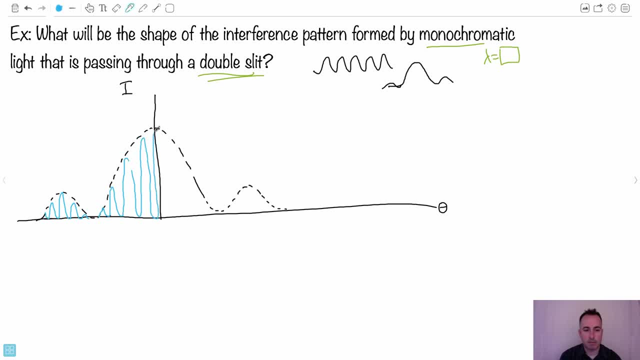 really high things right here, Probably have a peak right in the middle. No, it doesn't make that sound. Basically, you get the idea here. This is something here that's this kind of shape right here. Looks a little bit complicated, but you have to. 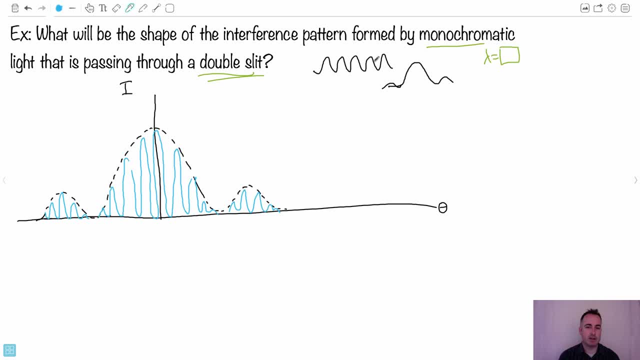 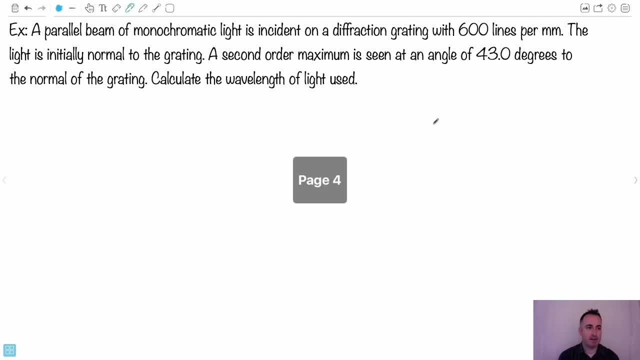 just think it's going to be a regular multiple slit diffraction thing that's modulated by a single slit. So this is the shape of it. I think it's kind of interesting. Then we have a real question here. Parallel beam of monochromatic. 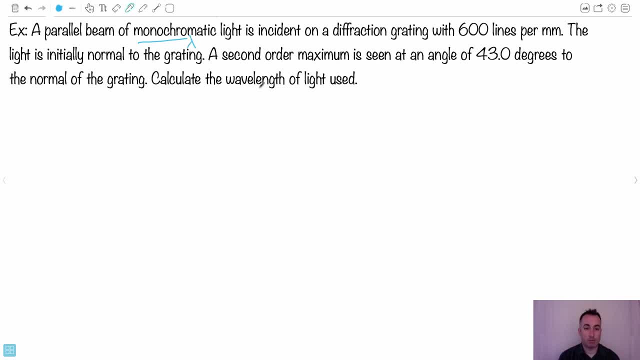 light. That means we can find lambda. Hey, that's the whole point of it. We're supposed to find lambda. It's incident on a diffraction grating. That means we have a situation like before. You know, we have a whole bunch of different holes here. We 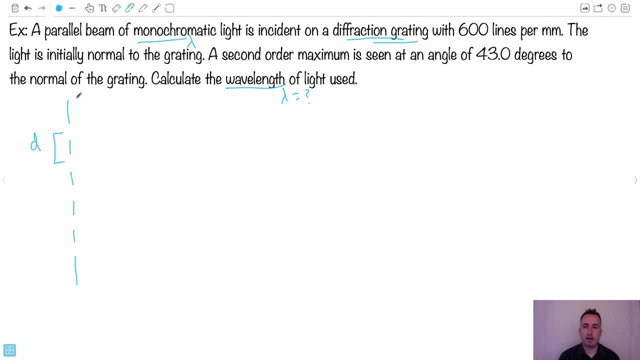 need to find this D, I guess. right, We're going to need to know that diffraction grating. We know there's 600 lines per millimeter. Now the light's initially normal to the grating, which means it's- you know this way here- like this, That's. 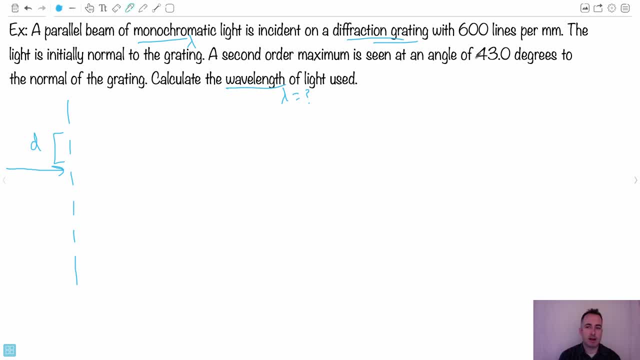 the way the light is And a second-order maximum is seen at an angle of this square. It's much to the normal. So what this means, then, is we have a second-order maximum, which, in this case, right here, let's see that's well. let's look at the 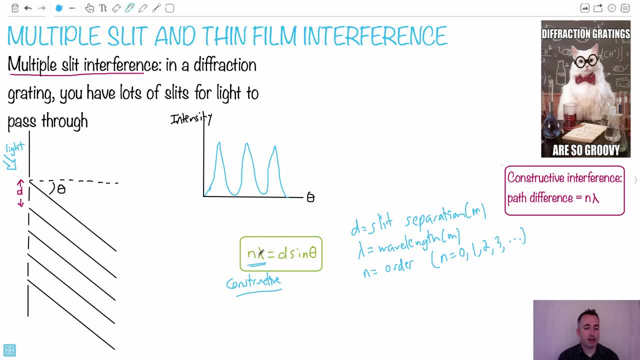 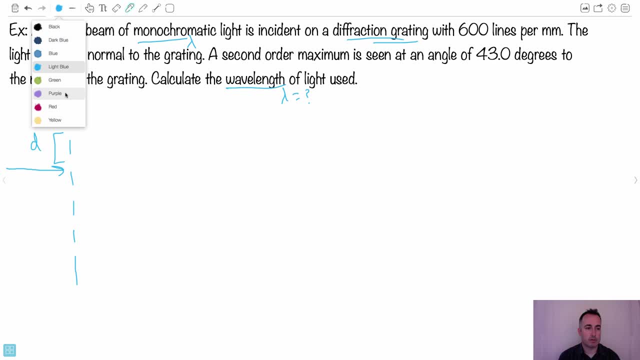 equation first. Maybe that'll help us. This equation here: n lambda equals D sine theta. We're going to need that. So n lambda equals D sine theta. Try to remember that. Here we go. We'll use n lambda equals D sine theta. n then will be. 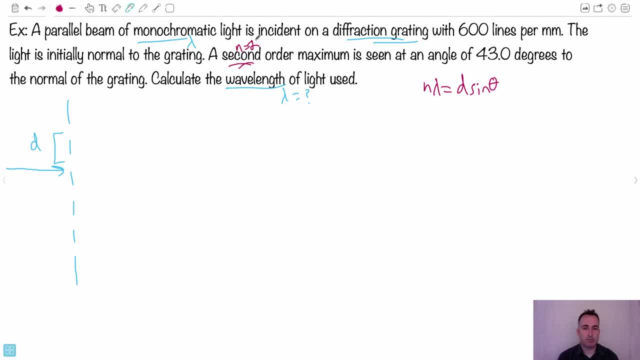 my, if it's second-order, that means n equals 2.. You're okay with that? That means then I can put in a two here. So 2 lambda equals D sine. and then theta's my angle, that you know where I see the maximum. So in this case, right here it's gonna be. 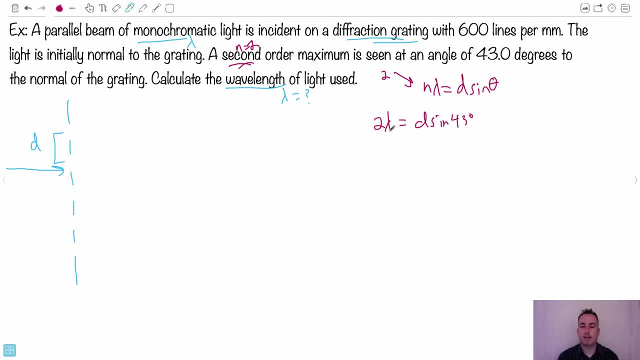 43 degrees And I need to solve for lambda. So that's gonna be pretty easy, right? So lambda is gonna be D sine of 43 degrees. all that divided by 2. Pretty easy, I just need to find D. See, that sort of tells me my mission Then is I need to 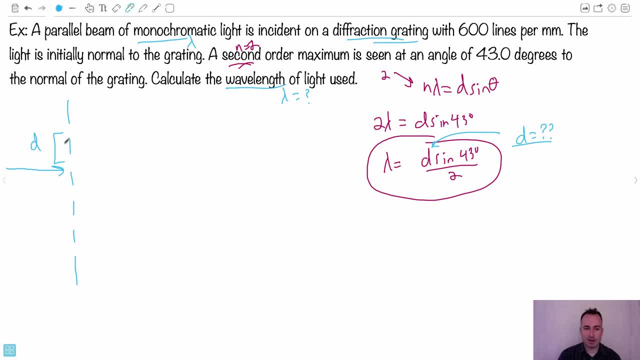 to find lambda. How will I get d? I need this distance right here. They've told us a bit of information here. Look carefully. They said there's 600 lines per millimeter. What does that mean? That means there are 600 lines like this per millimeter. I'm going to try. 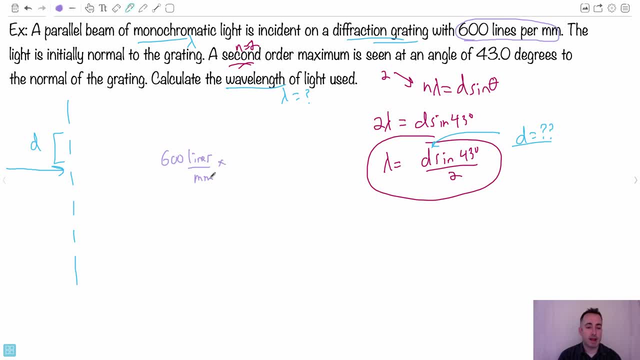 to convert that to meters. first I need things in meters. I'm going to try to get something that cancels out the millimeters. I'll put millimeters on the top, I'll put meters on the bottom. Do I know how many millimeters are in a meter? I do. There's a thousand. 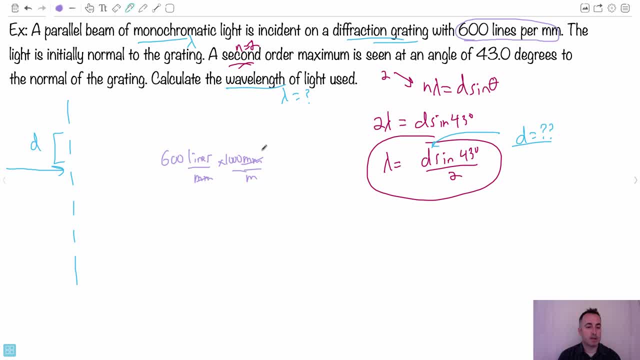 There's a thousand millimeters in one meter. That means the millimeters cancel out. Now I have 600,000 lines in one meter. This is going to be useful because I- I mean some people- we can actually call this capital N. That's one way to do it, but d is always one. 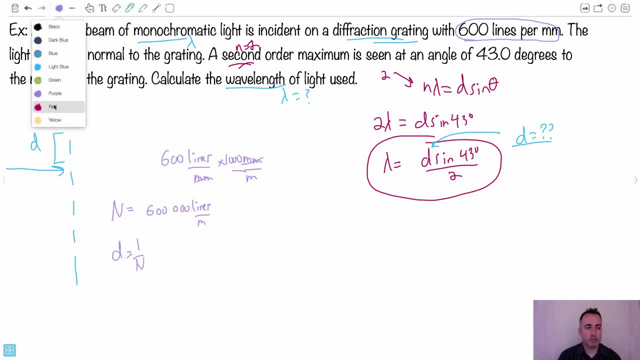 over N. This is actually maybe an important thing you might want to know about. I don't think you have to necessarily memorize it. If you look carefully at the units for it, it should work out. Let me show you something here. The reason why is because I need to. 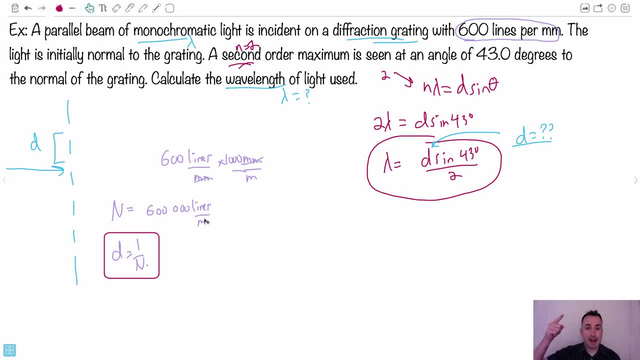 know this d in meters. Do you notice? here I have 600,000 lines every meter. I want how many meters per line, is it? If that makes any sense? I want to do one over this answer. That's why this d equals one over N, sort of came from. that Just says, well, all I could. 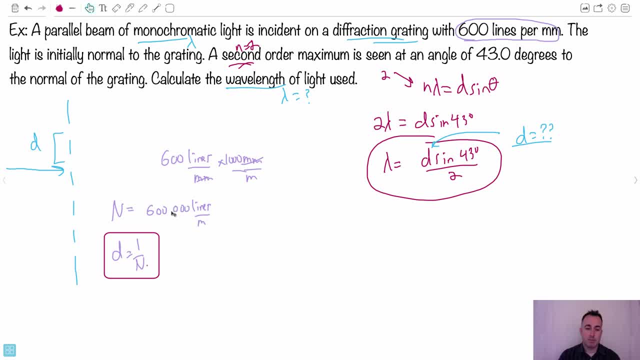 do is. I know the 600 lines per millimeter. I fixed that to meters, but I have to do one over that. How many meters per line? I needed it in meters, didn't I? I need a d in meters. That's why. 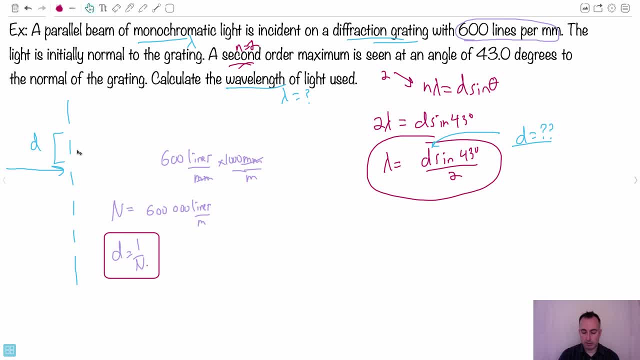 I do one over 600,000.. Oops, too many zeros. I end up with an answer of d equals- Hopefully you're following with me here. I end up with that d equals 1.66, repeating obviously, I'll say 1.67 times 10 to the minus 6 meters. It should make sense If you have 600,000 lines. 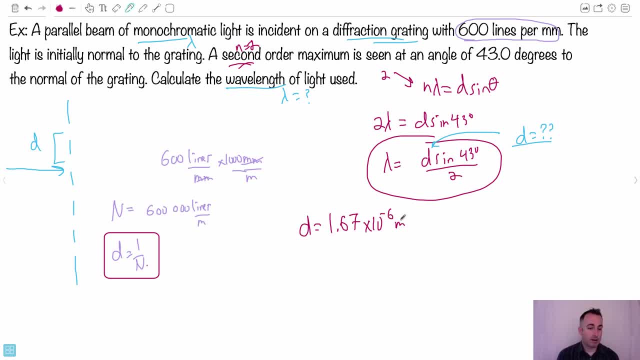 in one meter. it should make sense. You have not many meters for one line. It should be a very, very small number. I plug that into here, so I end up with. Maybe I'll do it in a different color Before I.